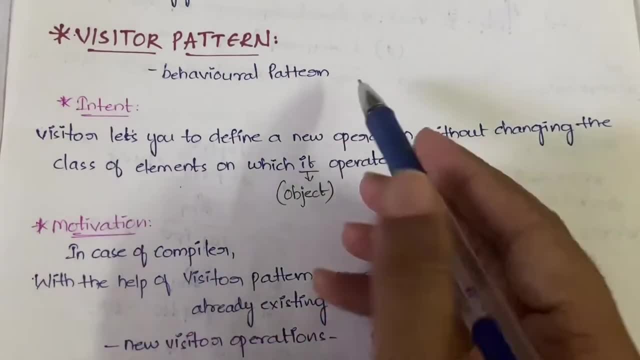 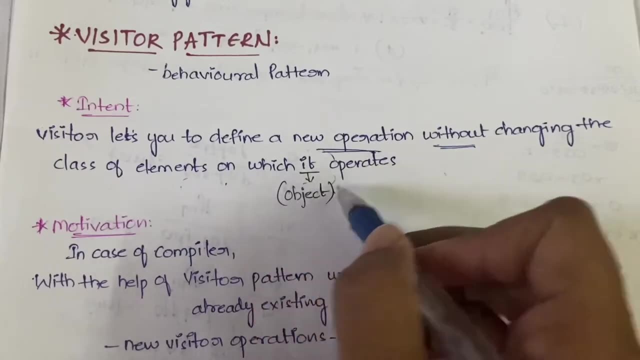 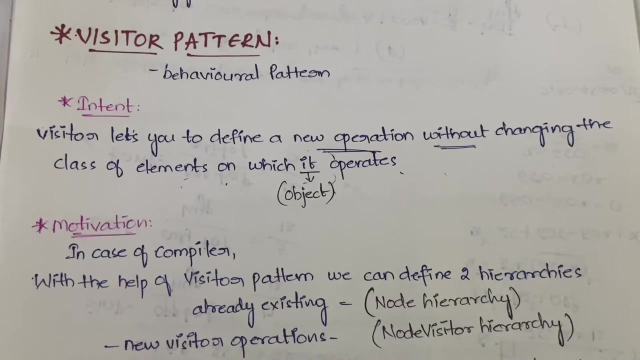 on which it operates. Visitor will let you to define a new operation even without changing the class of elements on which the particular object is operating. So you can, simply, we can say that you can define the new operation without changing the existing functionality, without changing the existing class, so that the other functions or other operations will not be disturbed. Okay, this is about the intent of the visitor pattern. 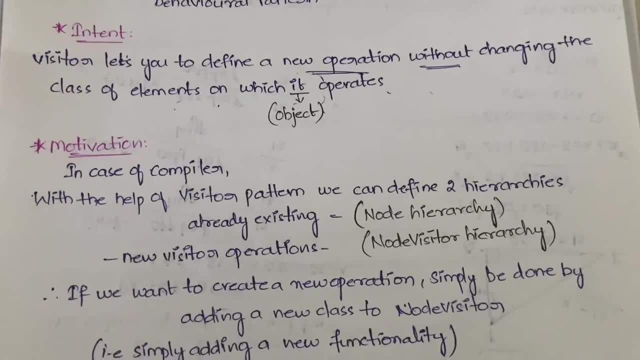 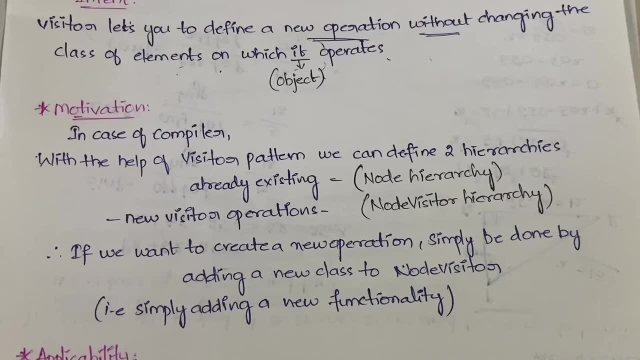 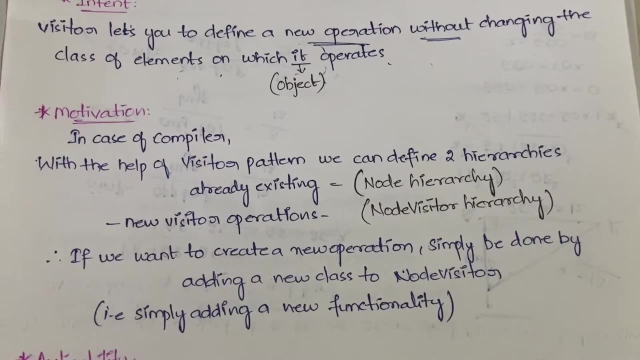 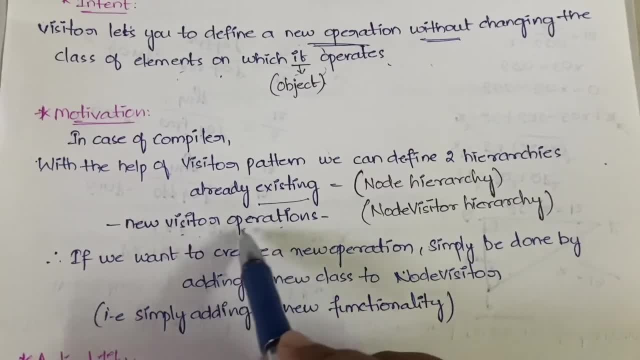 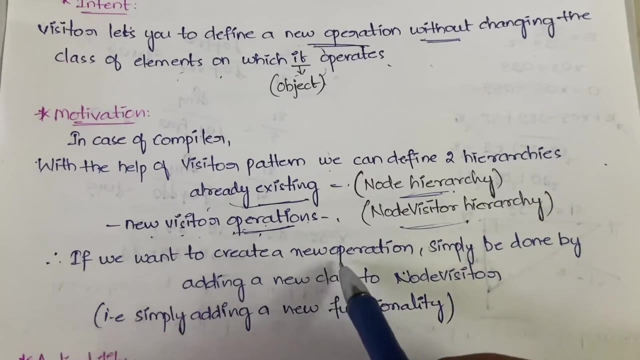 for already existing operations and the other one is for the new visitor operations, that is, newly coming operations. so for the already existing operations you are defining a node hierarchy, and for newly coming operations you are defining a node visitor hierarchy. got it so here? what happens is so when you are, when you want to create a new operation, you can simply how you can do that by: 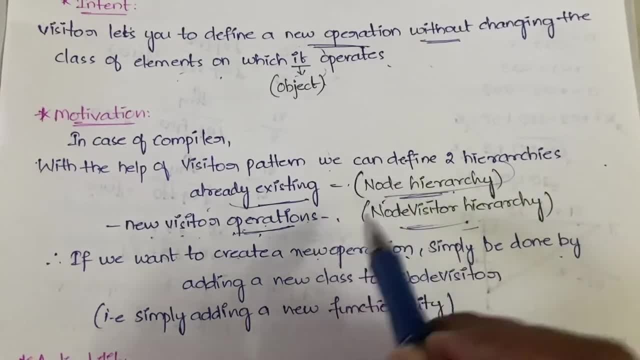 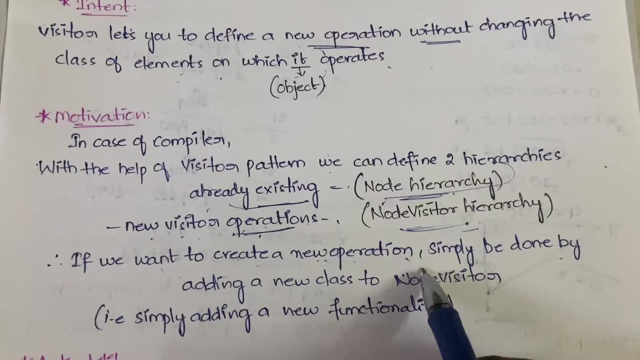 adding a new class to the node visitor. so node hierarchy is: we already have that. we already have a predefined existing um, you know, hierarchy or node hierarchy. you are now again defining a new hierarchy, that is node visitor. hierarchy right, create a new operation. so when you, whenever you, 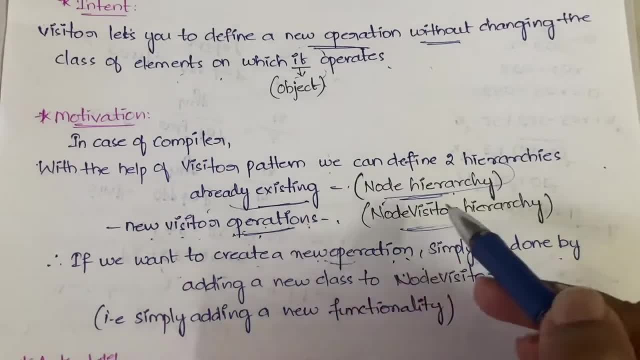 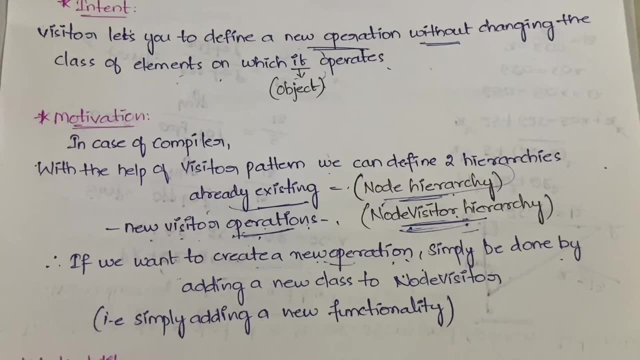 want to create a new operation, you can do it by simply adding a new class to this node visitor. instead of modifying the existing classes, instead of disturbing the existing classes, you can simply attach a new class and you can add a new functionality or a new operation. okay. 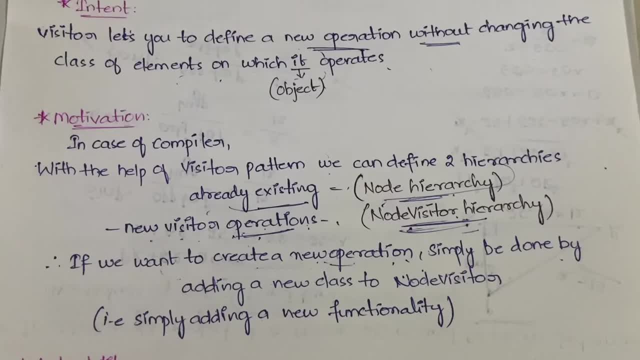 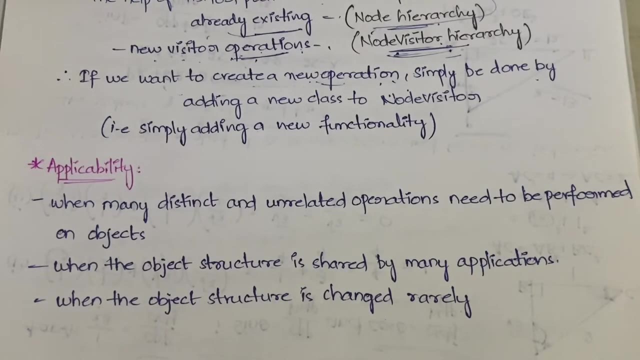 so that is simply adding a new functionality. got it. so this is the use of visitor pattern. got it. with the help of visitor pattern, you can easily add it, easily add a new operation. got it. now, moving over to the applicability of this, when many applicability in the sense you know right, when you can use this. 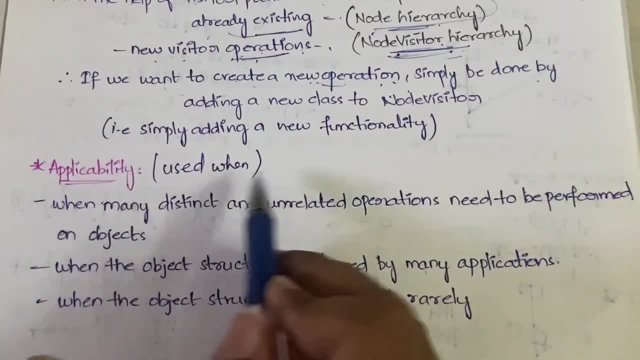 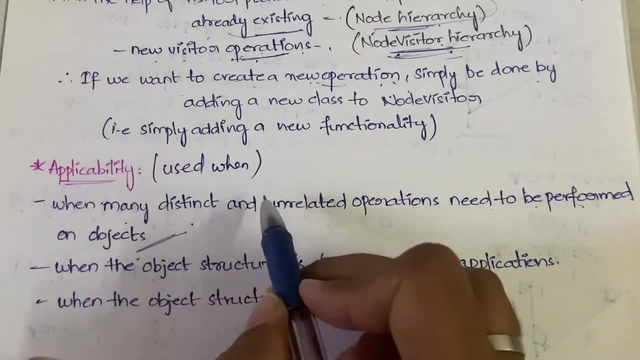 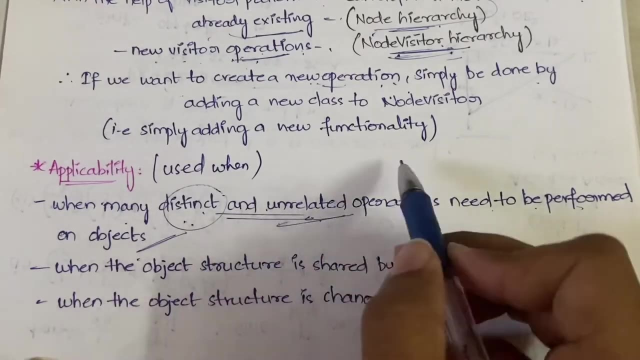 used when it is used when many distinct and unrelated operations need to be performed on objects. when you are have to perform many distinct and also unrelated operations- distinct in the sense, different, unrelated in the sense each one is not related to one another- you have to perform these kind of operations on the object. then 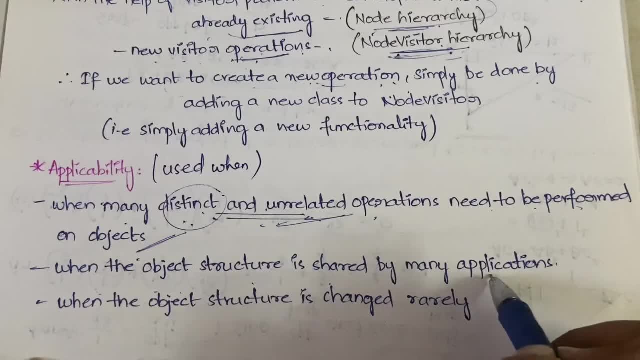 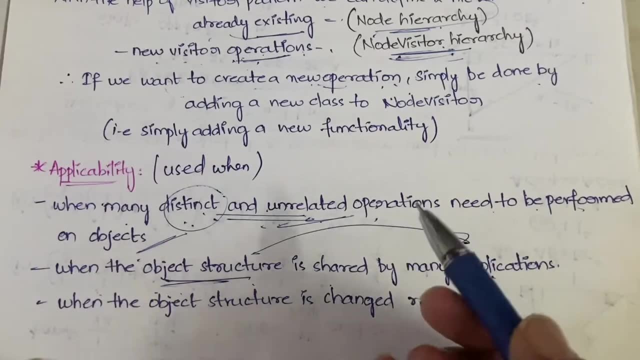 you can go for visitor. then the object structure is shared by many applicants. okay, single object structure is may is shared by many applications or just shared by many users. in that case also, you can use this. then the object structure is changed daily, that is once in a while you're. 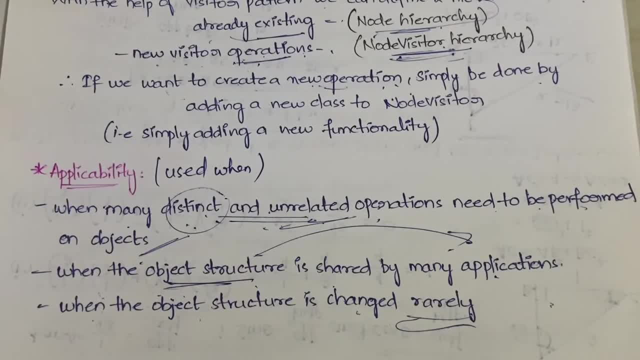 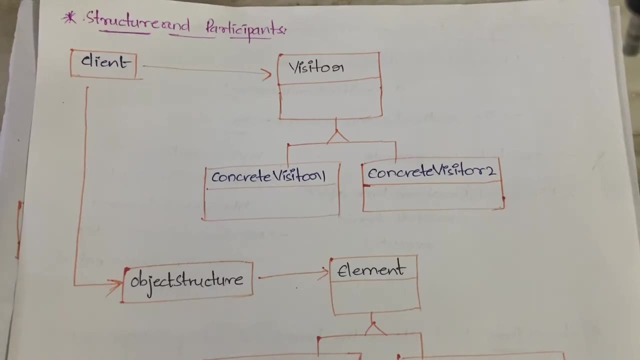 changing it not. you're not changing it rapidly, you're not changing it frequently. in that case, you can use this visitor pattern. got it. so this is about the applicability. till now, we have discussed the intent, motivation and also applicability right now. structure and participants of visitor pattern. so the structure is a bit longer. 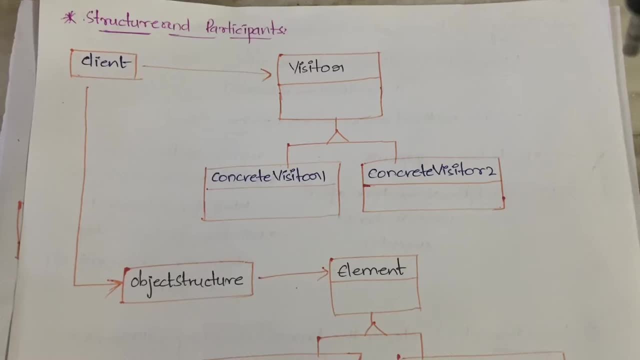 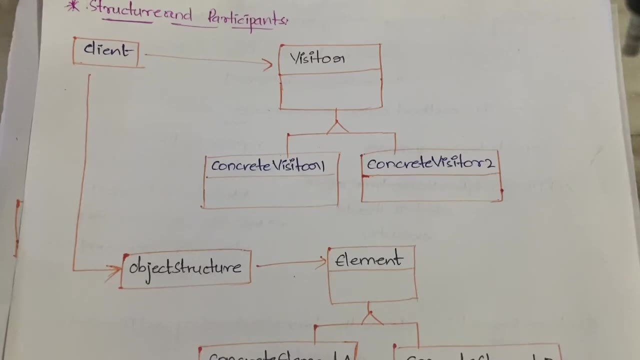 so you need in the exam, when you're writing it, you need to keep the heading as structure and draw this, and then again, below this, you have to write a heading- participants, and you need to describe each and every participant which you have drawn. got it, so now let us see what. 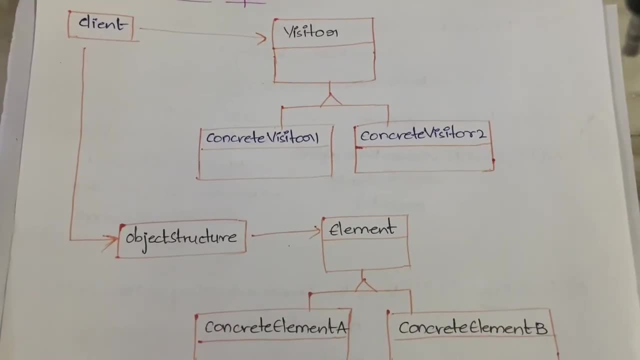 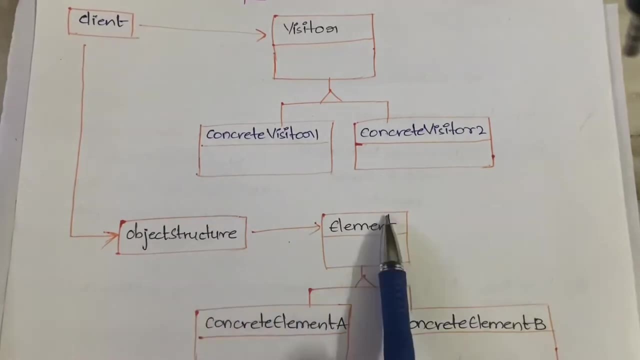 does the structure and what are the participants involved? okay, see, it has. what are the, what is the structure, that is the structure and what are the participants involved? visitor- concrete visitor. object. structure element, concrete element. got it. now let us see what each will do. first, we have is a. 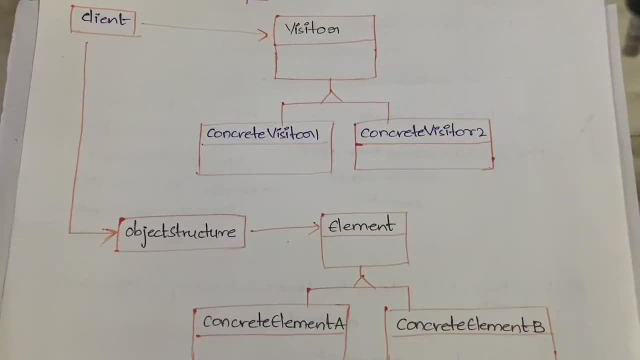 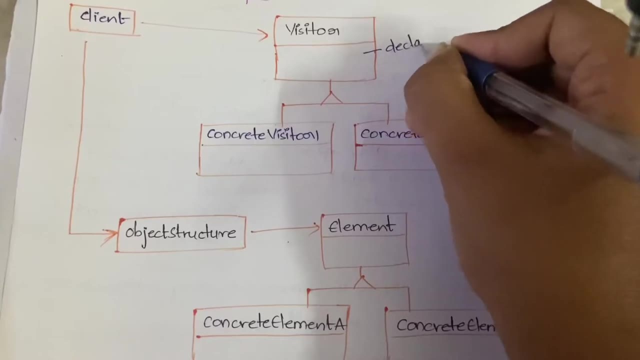 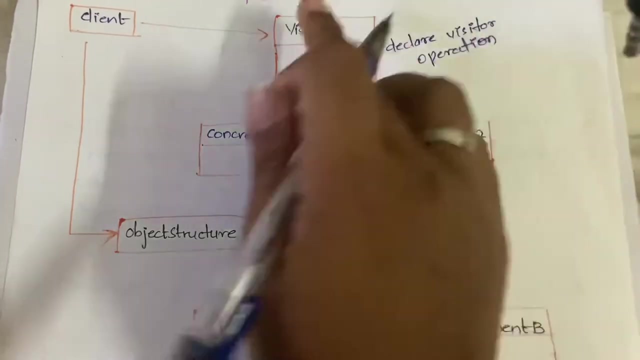 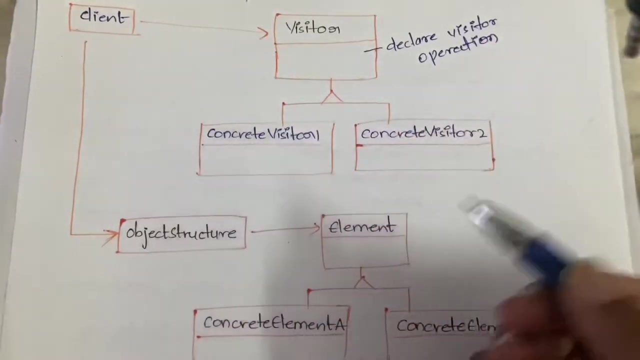 visitor right. what visitor will do is the visitor. it will declare a visitor operation for each class. what the visitor will do? it will declare a visitor equal to관 operation. got it. so the visitor will be declaring the visitor operation. then what do we have? concrete visitors. what concrete visitors will be doing? it is very obvious. we have been learning. 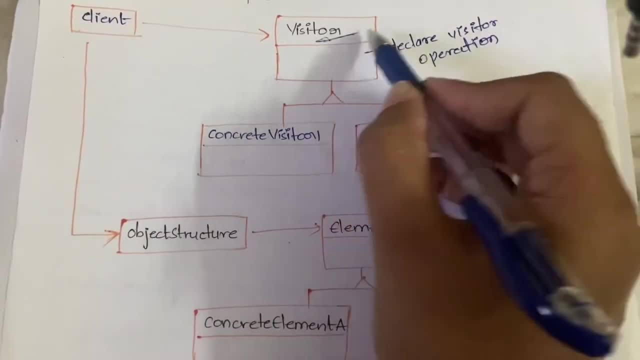 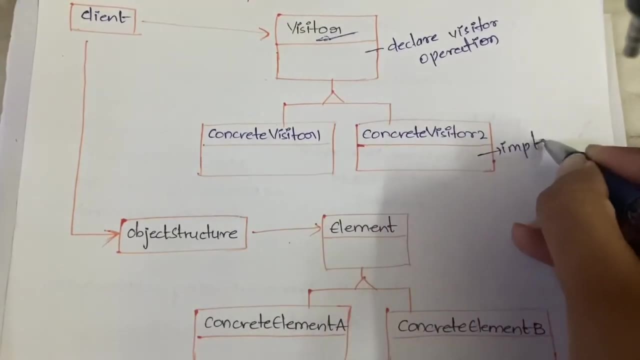 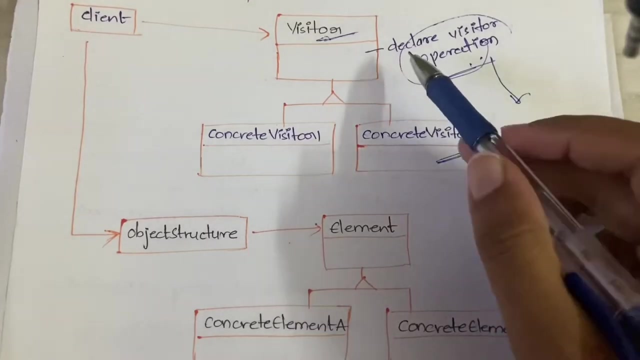 from so many design patterns. the visit, the main thing will be declaring the concrete ones will be implementing. so the same will happen even here also it they will implement the. so whatever is declared here or whatever is defined here, that will be implemented by the concrete visitor. so here, what we are doing, we are declaring the visitor operations, right here. 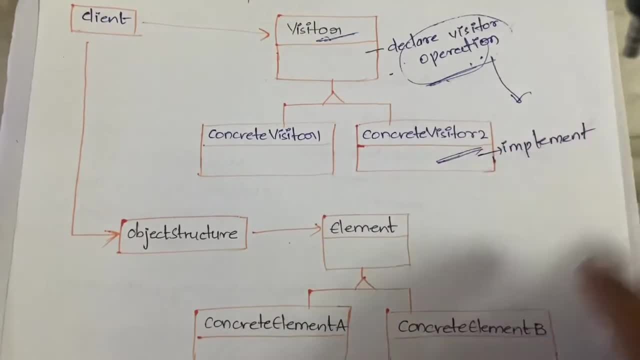 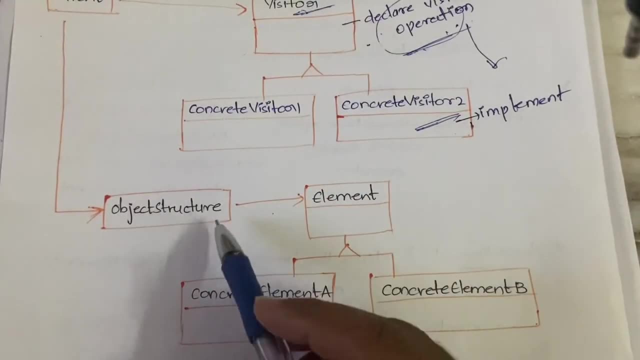 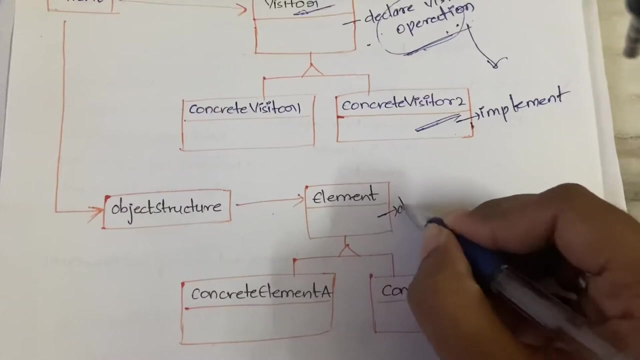 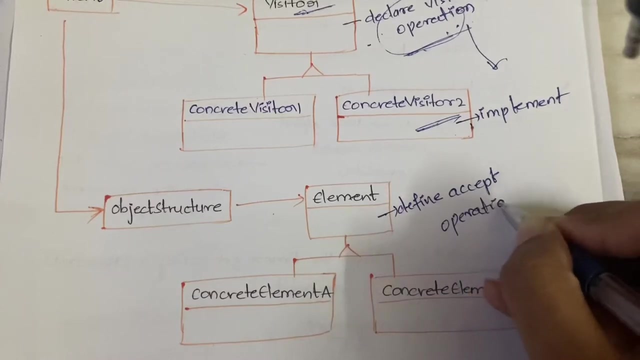 the visitor operations will be implemented. got it now. after visitor and concrete visitor, what do we have? we have the object structure element and concrete elements. right now. what this element will do: element will define an accept operation. so it will define accept operation. got it. what do you mean by this accept operation? 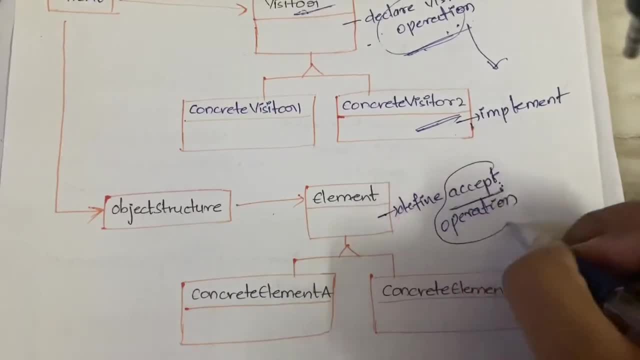 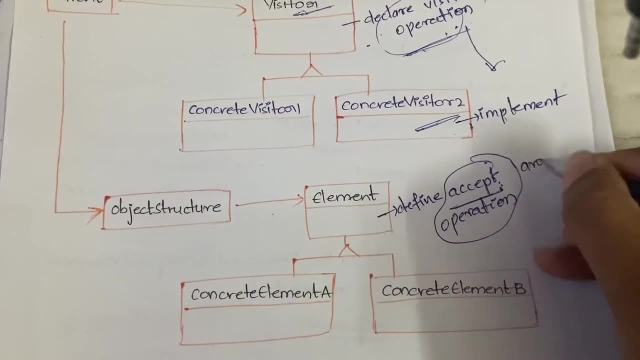 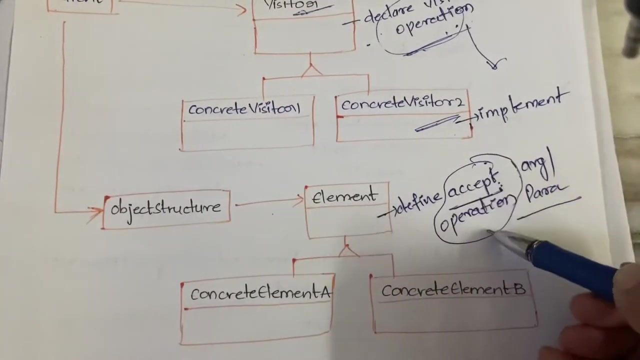 means i'll tell you this will take this accept operation. what it does is it will take the visitor as an argument. okay, as a parameter. you can say as a argument or as a parameter, like according to your convenient. okay. so here the element is defining the accept operation and what this? 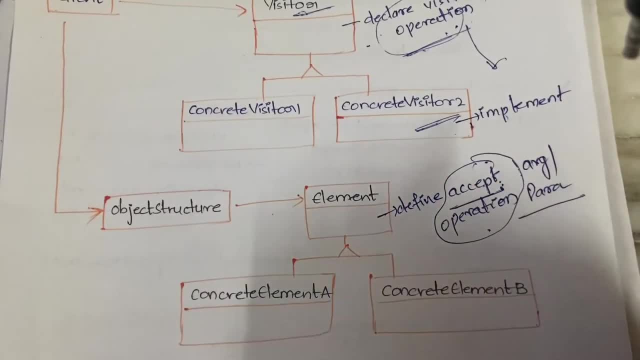 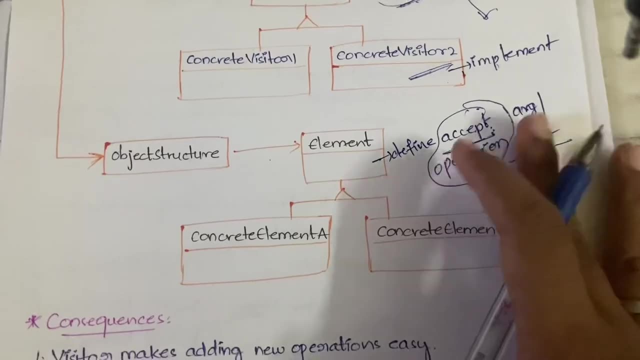 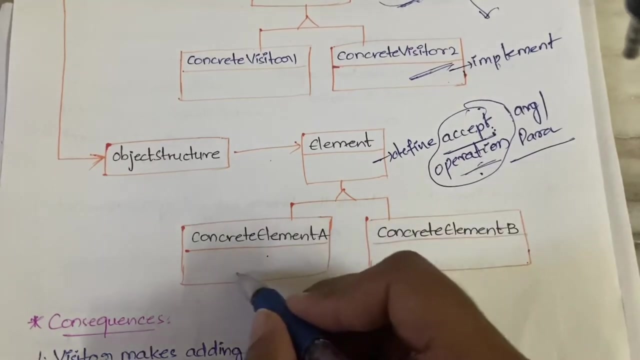 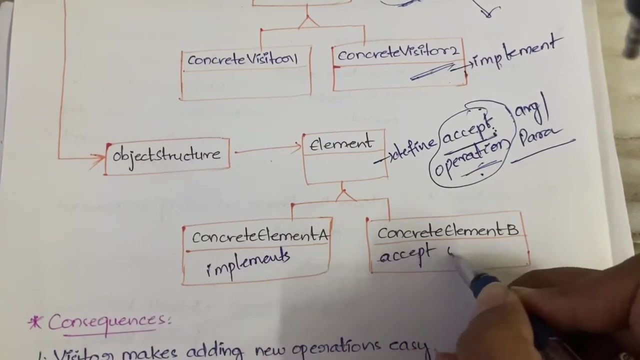 accept operation will do. it will define the argument or parameter. right visitor will be declared as an argument or parameter that you have to remember here. got it now after the element. what do we have? we have the concrete elements. right again, same here. the accept operation is been defined. here the accept operation will be implemented. implements accept operation. 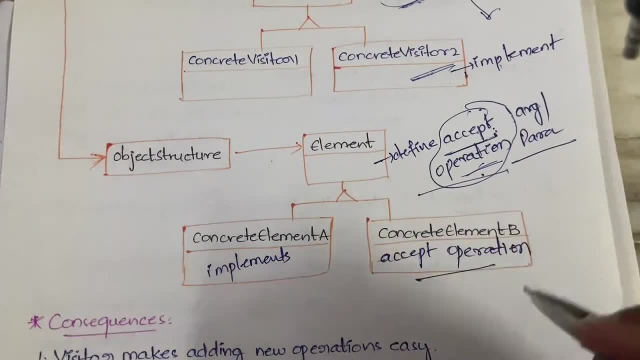 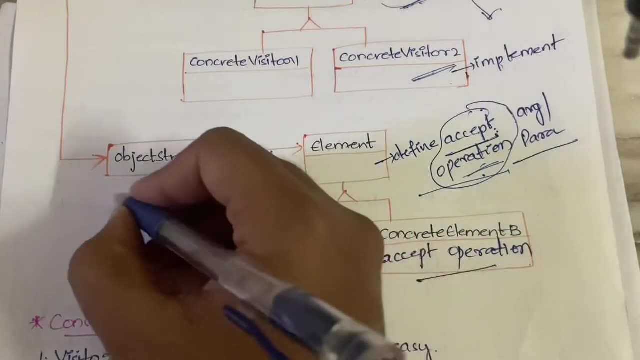 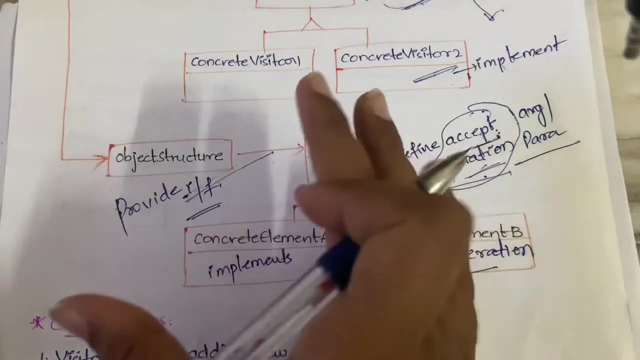 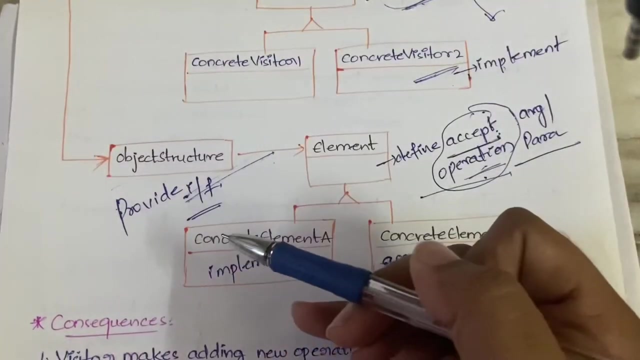 got it here: definition here, implementation next, what is left? object structure is left. what object structure will do is it will provide a high level interface. it will provide an interface that to a high level interface to allow the visitor to see its element. right. we have the visitor pattern right. the visitor pattern can see its elements, it can visit its elements. 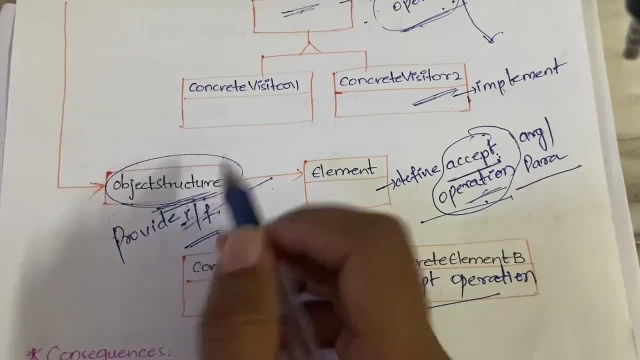 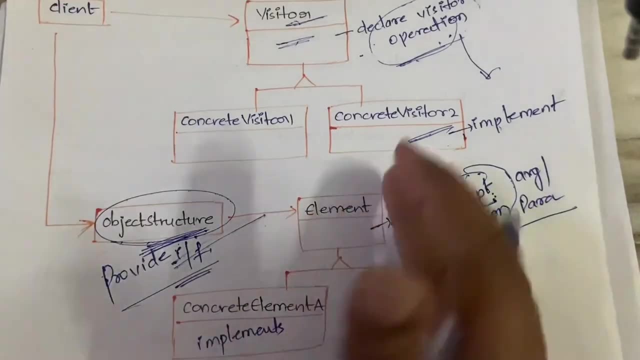 through the interface which is provided by the object structure, the visitor pattern and the element are linked to one another with the help of this object structure. it provides a high level interface through which the visitor pattern can view or can see its elements. got it so this is. 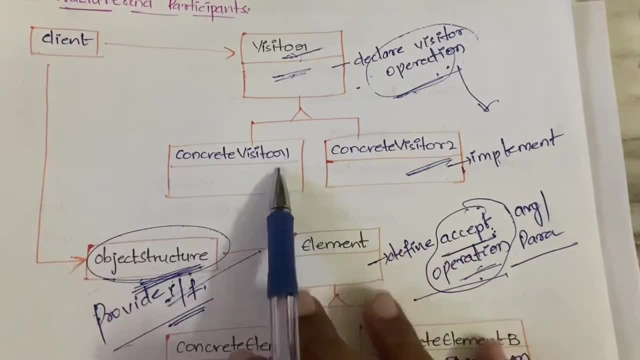 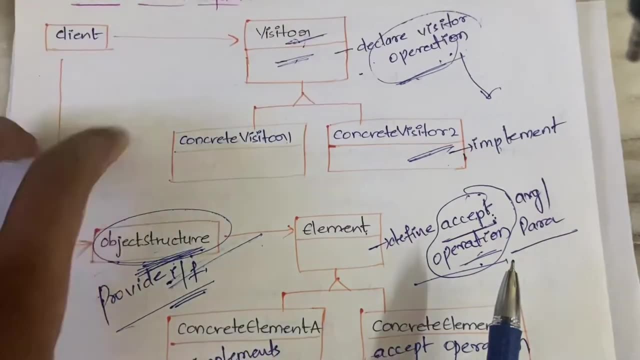 about the structure. in structure we have visitor- concrete, visitor, element- concrete element and the object structure. object structure is nothing but it is an interface between the visitor and the element. got it. and what visitor will be doing? it will be declaring the operations and what concrete visitors will be doing. they will be implementing the operations declared by the. 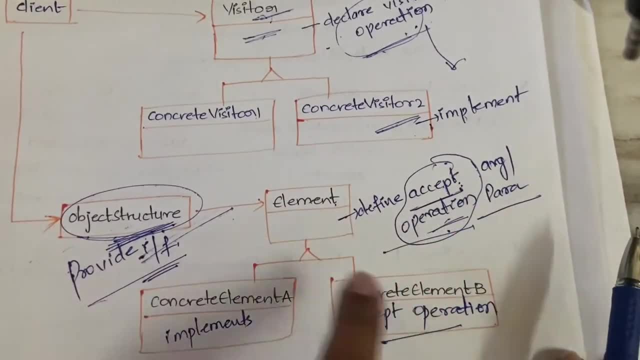 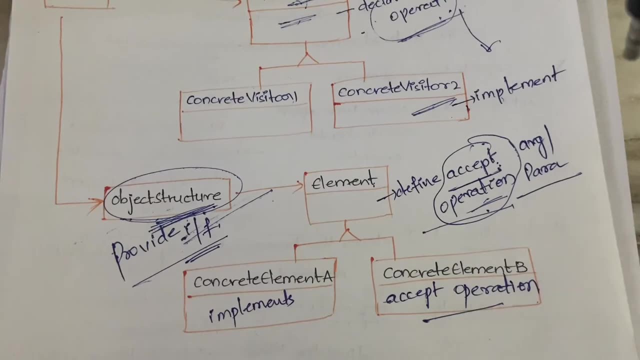 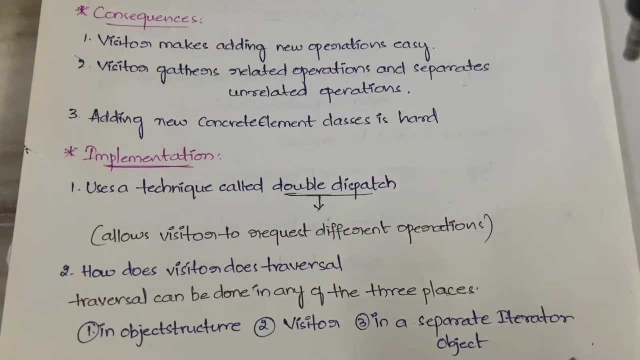 visitor, what element will do? it will define the accept operation and concrete elements will be implementing this accept operation. that's all very simple. got it now done with the structure and participants. now let us see the consequences and implementation, followed by new users and also related patterns. with that we can end this video. so consequences. 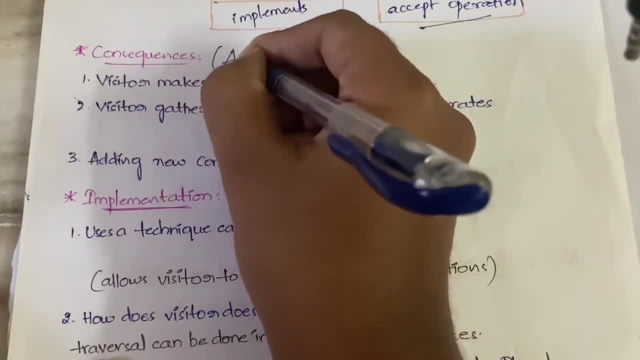 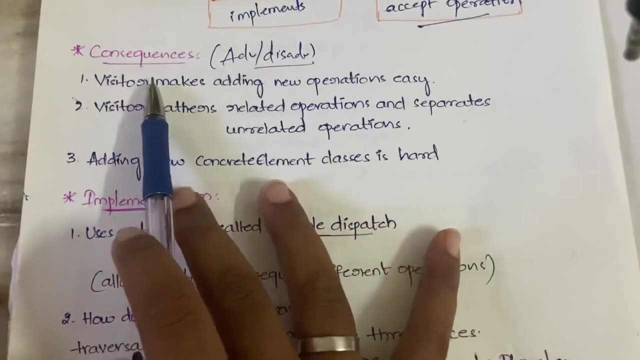 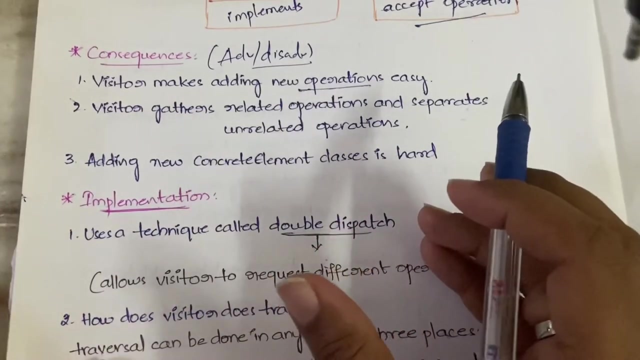 means you know right consequences means it can be either advantages or disadvantages of using this visitor pattern. so let us see we have three. visitor makes adding new operations easy. obviously, because when you want to add a new operation you need not do any disturbance to the existing operation. you 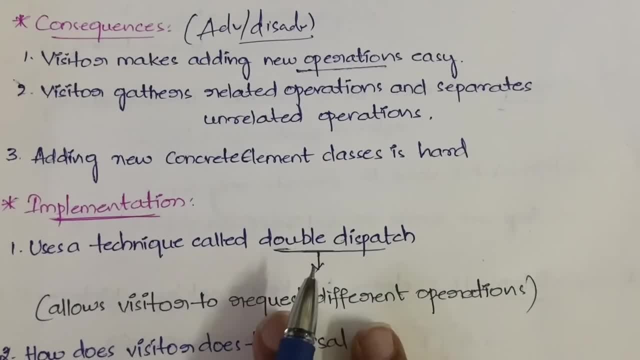 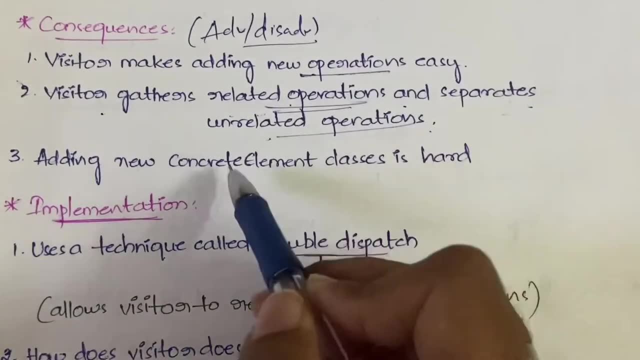 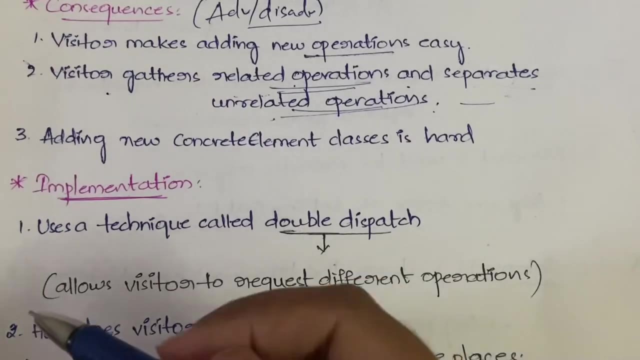 can automatically add it very easily: right and visitor gather. related operations and separated separates unrelated operations. related operations will be grouped together and unrelated operations will be grouped together, by which you can do the operations very easily, by which the operations can be implemented very easily. okay, and third, adding a new concrete elements. 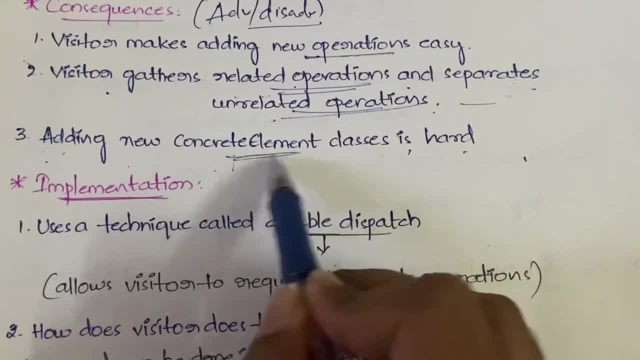 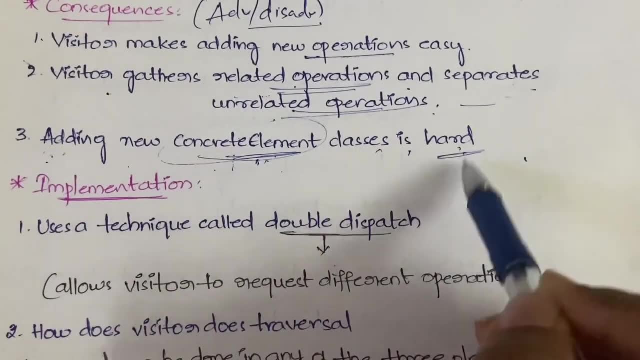 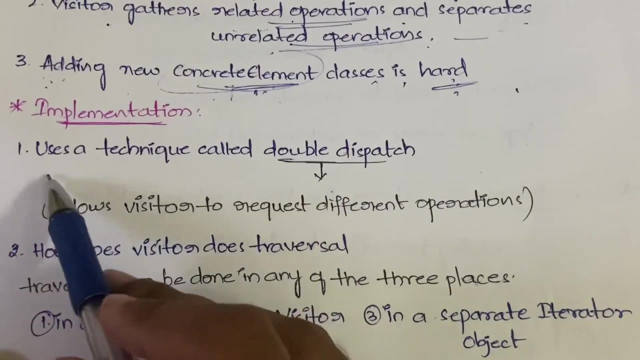 classes is hard. so you know what concrete element is that it will be implementing the accept operation. so adding a new concrete class is a bit difficult in case of visitor. okay, got it. next implementation. so in implementation, let us see what do we have. it uses a technique called as double dispatch. so what do you mean? 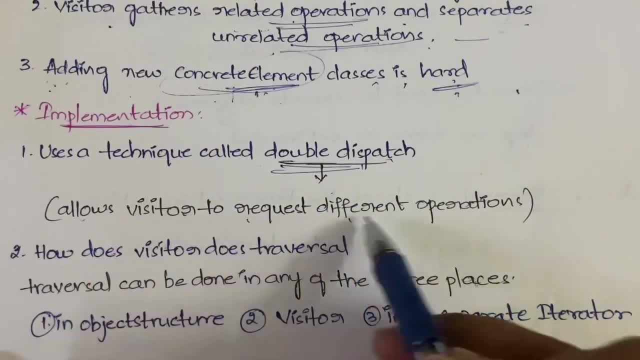 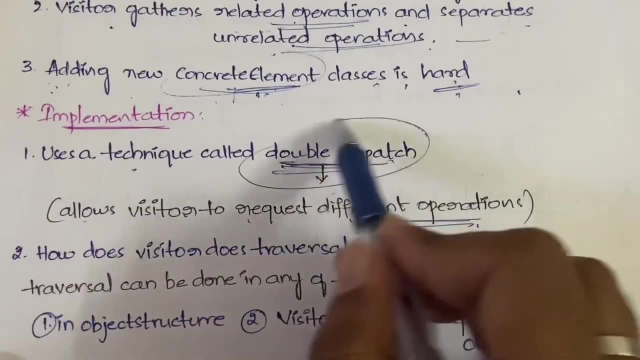 by this double dispatch, i'll tell you. it will allow the visitor to request different operations. so, with the help of a double dispatch- here you are using a technique which is called as a double dispatch, double dispatch- with the help of double dispatch, what you can do, it will allow the visitor. 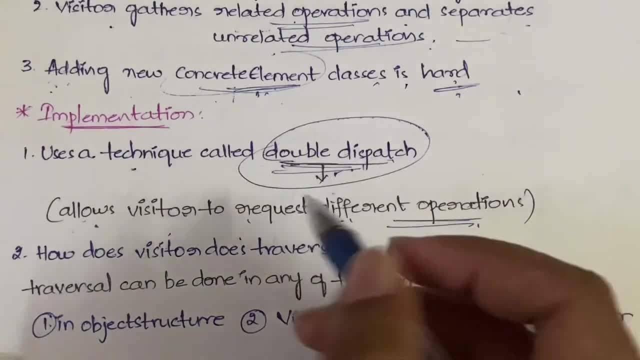 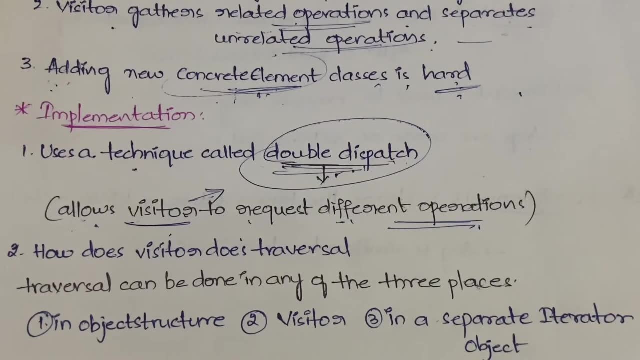 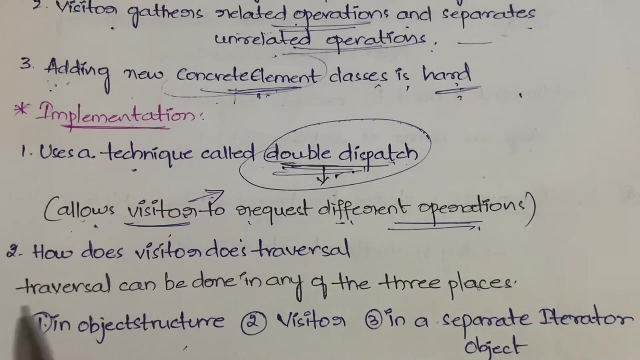 to request different, different operations. so a single visitor pattern can perform multiple operations. can support can be used to- uh you know, add classes for multiple operations with the help of this double dispatch method and how visitor will do the traversal, that is how a visitor will be approaching its elements, so it can be by object structure, which we have seen in the structure. it. 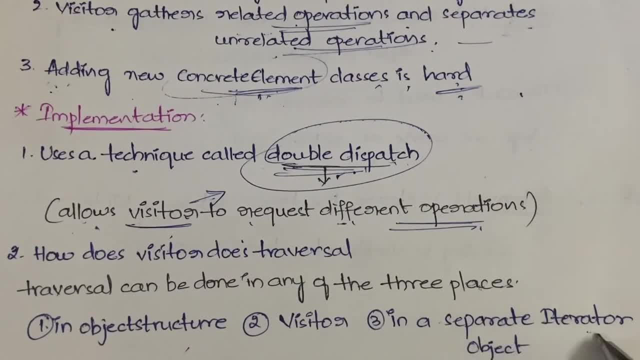 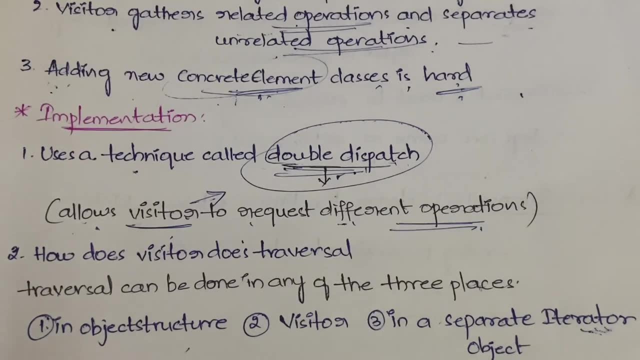 can be directly through the visitor or it can be through a separate iterator: object. okay, got it. so this is about the implementation. got it. so: visitor, how it can see its elements, how it can approach its element by three ways: by the object structure, or by visitor, or by the separate.